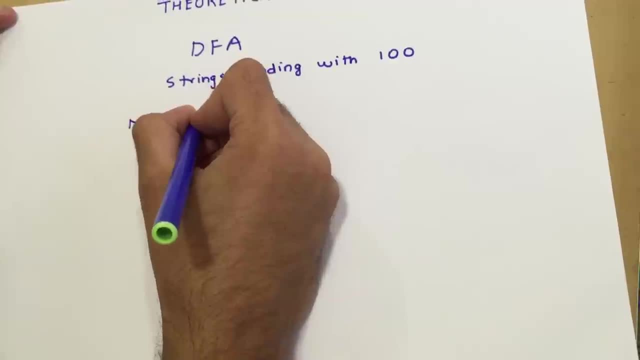 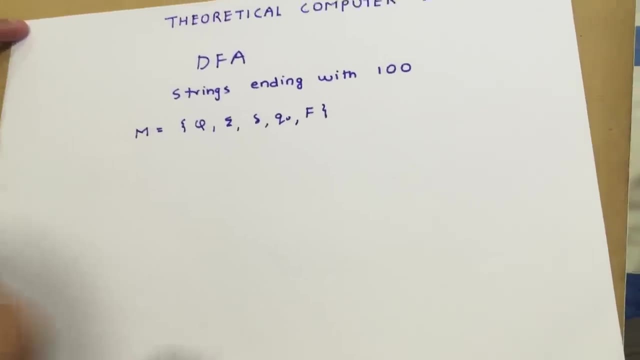 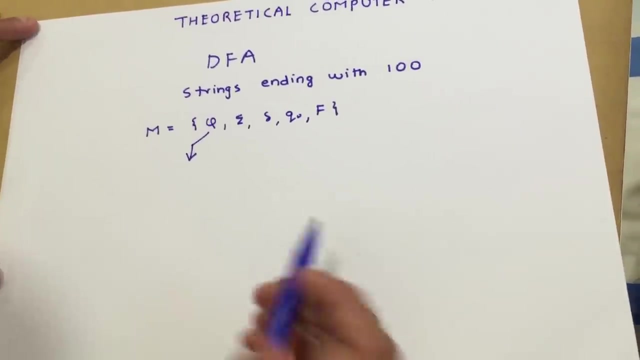 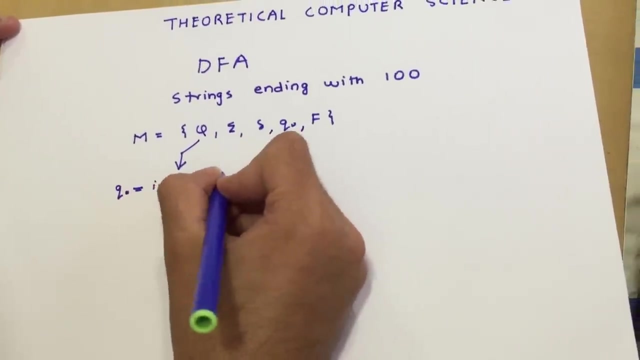 make the mathematical model. The mathematical model is Q sigma del Q 0, f. So now for the Q part. So I am going to take four states. How to take the states, I am going to teach you now. So first I am going to take the initial state, Q 0, and I am going to take a state Q 1 for 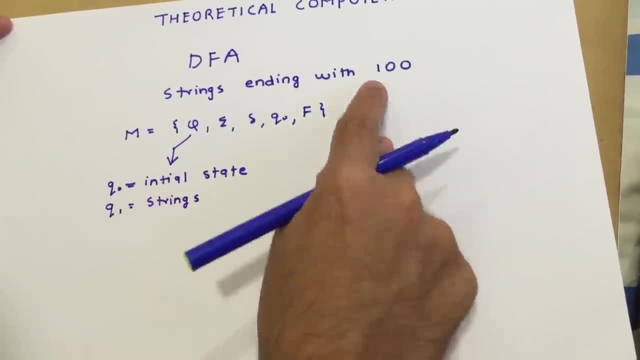 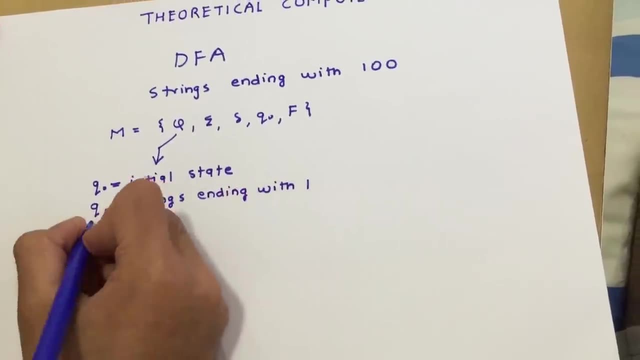 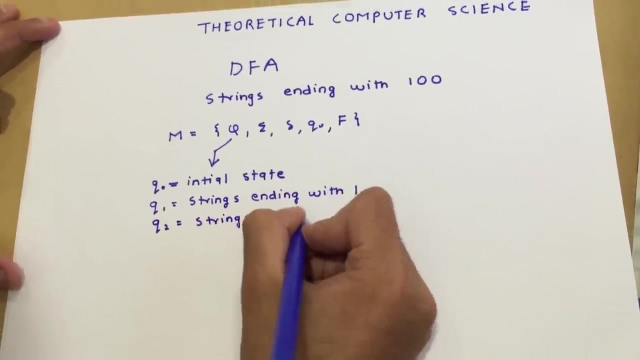 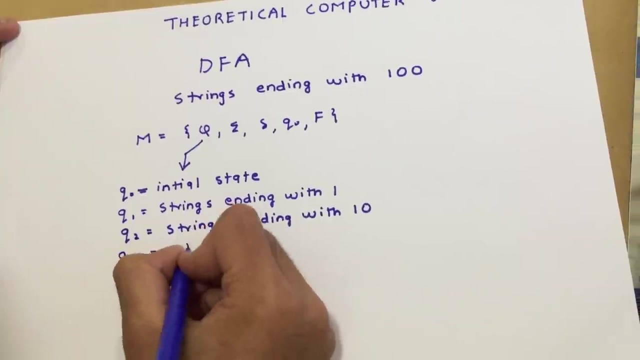 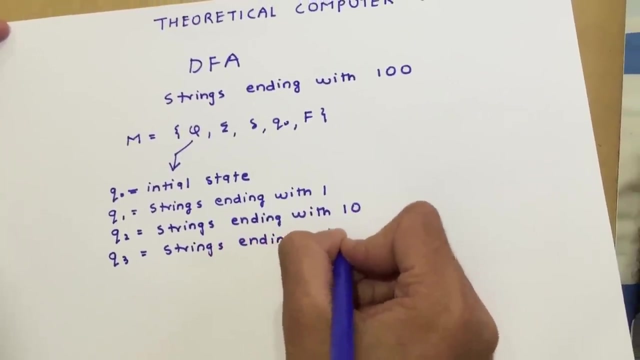 strings ending with 1.. Then I am going to take a state Q 2 for strings ending with 1.. Strings ending with 1- 0. and the last state Q 3: strings ending with 1: 0- 0.. So I am going. 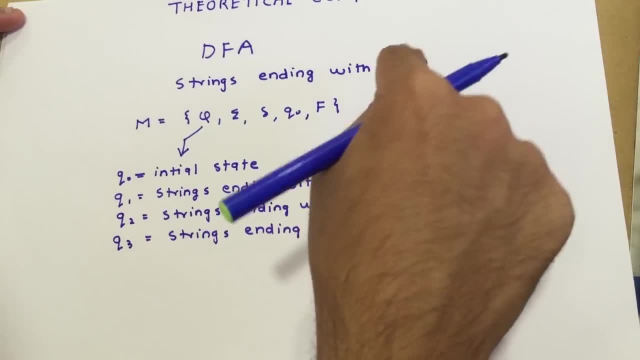 to take three states. Depending on this, you can take these states: initial, ending with 1, ending with 1: 0, ending with 1 0, 1.. Now, as we know, our input alphabet is 0 1, 0.. So 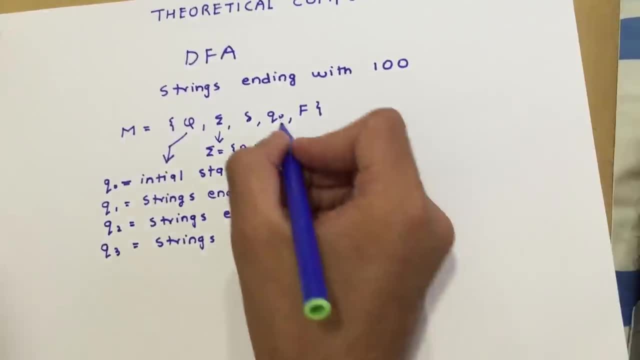 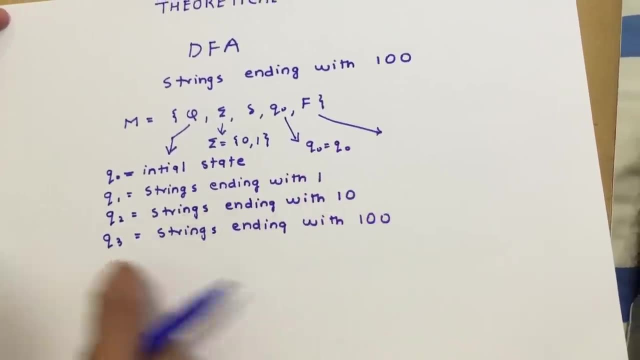 our input alphabet is 0- 1.. My Q 0 is going to be Q 0 and, of course, my final state- as you want strings ending with 1 0, 0- is Q 3.. Our final state will be our final state will. 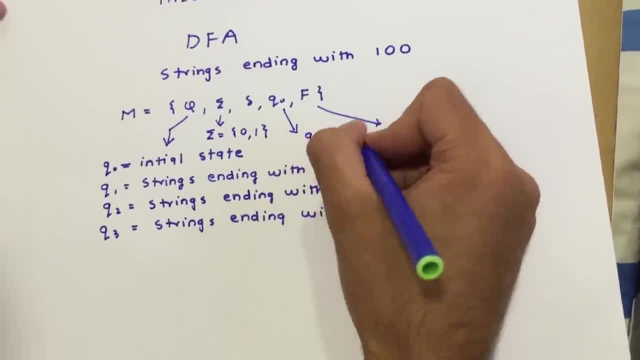 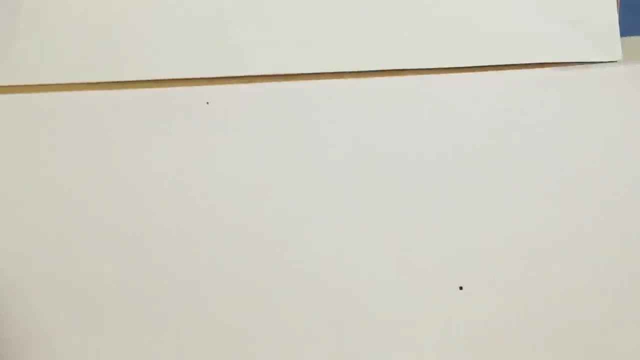 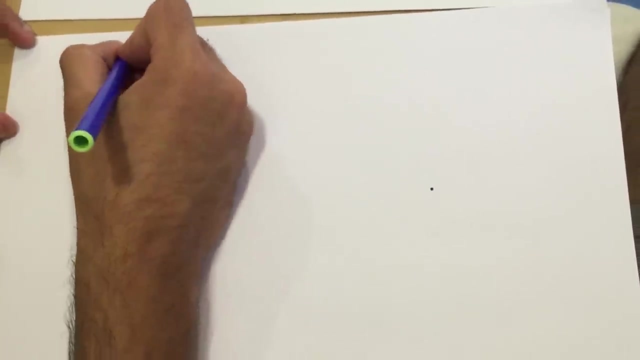 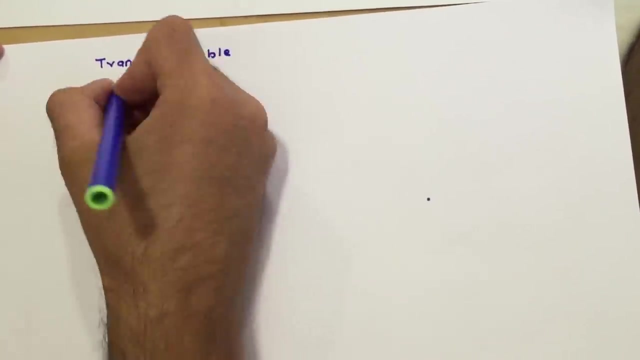 be Q 3.. Now all we have to, all we have left, is to calculate the transition function. So I am going to start calculating transition function. I am going to do that with the help. First, I am going to draw a transition table. So how to draw a transition table? So what? 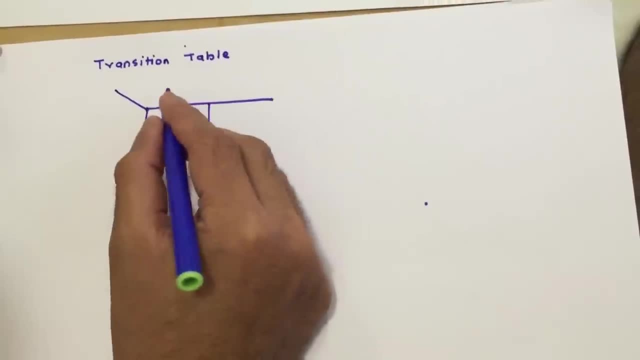 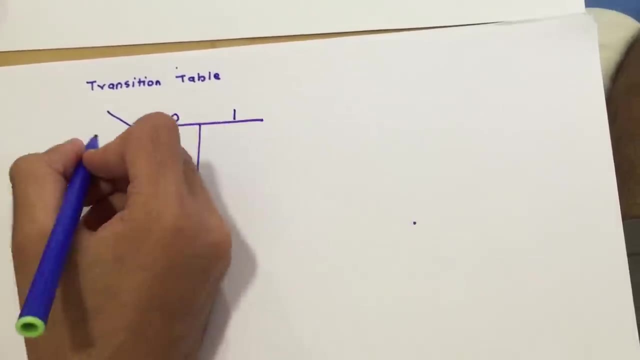 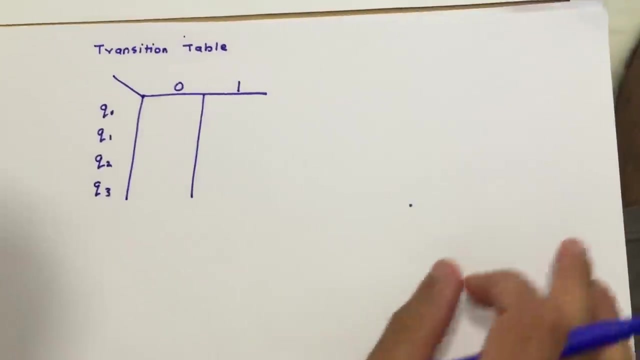 we do is on this side we write all the states, and on y axis we write all the states and on x axis we write all the input alphabet. So I am going to write 0 and 1 here, and q 0,, q 1, q 2 and q 3 here. So, guys, this is where the new method comes in. This is a little. 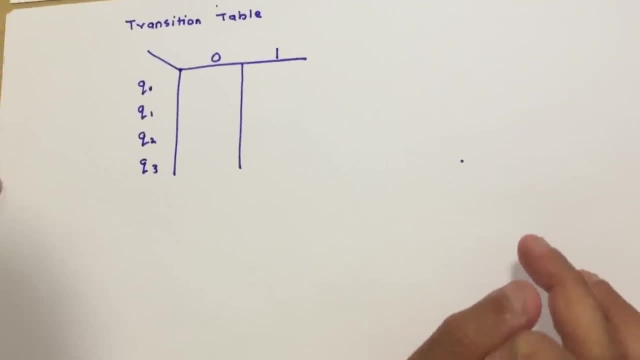 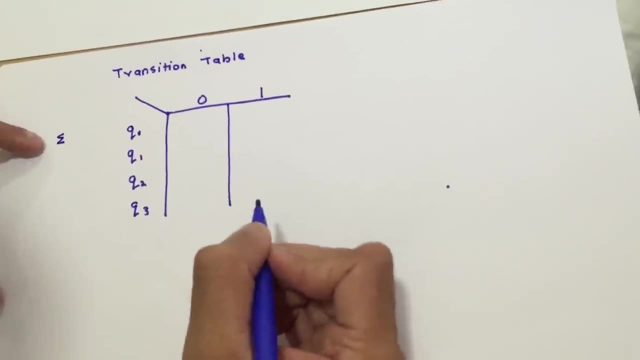 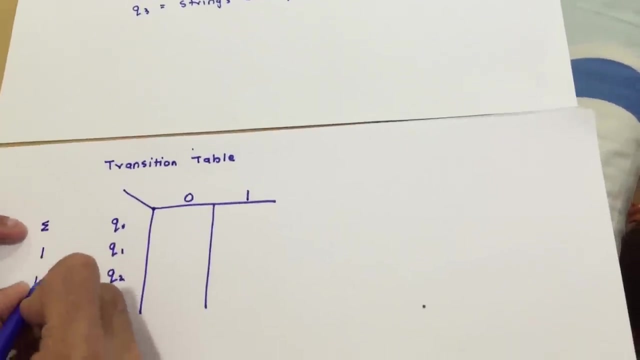 different, but all the problems become really easy to solve. So now what I am going to do is, since this is the initial state, I am going to write an epsilon beside this. Since q 1 ends with 1,, I am going to write a 1 here For this. similarly, I will write a 1, 0 and. 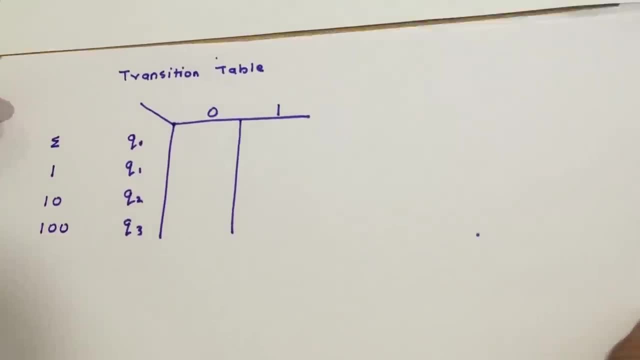 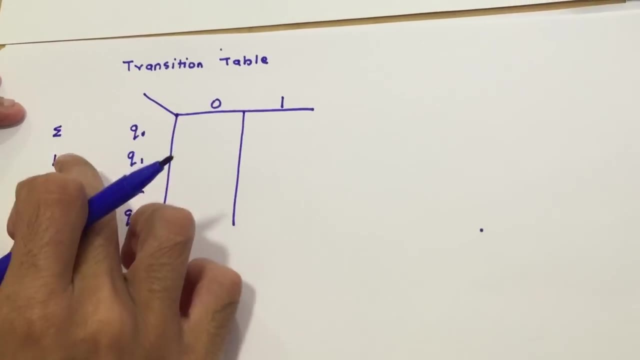 for this, I will write a 1 0 0.. So what I am going to do is I am going to write a 1 0 0.. So what I am going to do is I am going to consider these two simultaneously and see if that lies within our states. For. 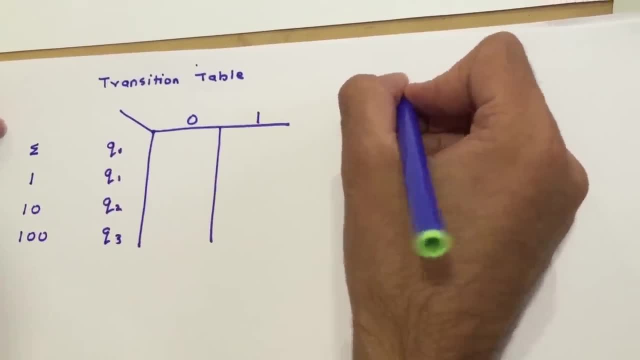 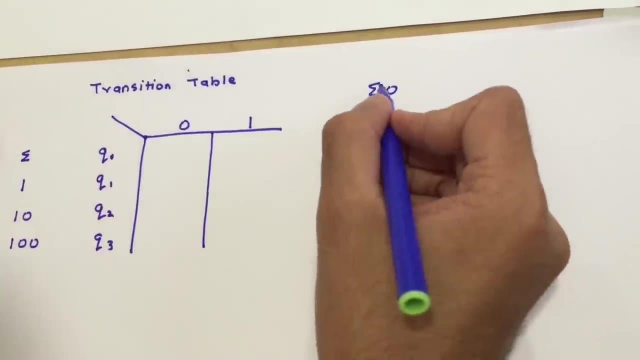 example. first I am going to consider sigma 0.. Can we see sigma 0 anywhere here? No, Sorry, epsilon 0.. So is there epsilon 0 anywhere here? No, So I am going to first cut my epsilon. 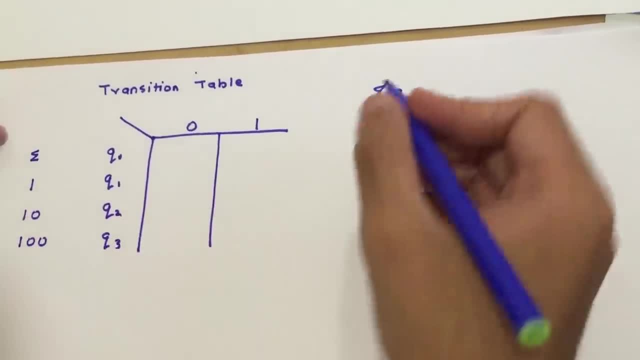 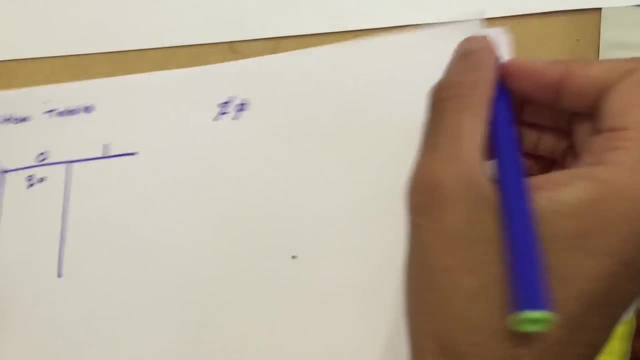 then I check 0.. Can I find 0 anywhere here? No, right, So I am going to cut this. If all states are cut, then we send it to q 0.. Similarly, I am going to do it for epsilon 1.. Is epsilon 1 available anywhere? No, So I am going to. 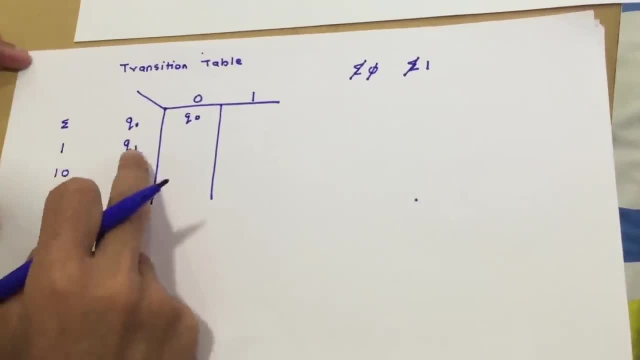 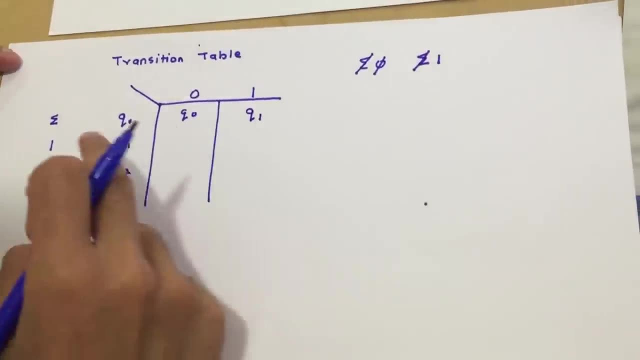 cut the first one. Is 1 available? Yes, And 1 corresponds to q1.. So when q 0 encounters 1, it should go to q 1.. Similarly, I am going to do this for all others. So here I am going. 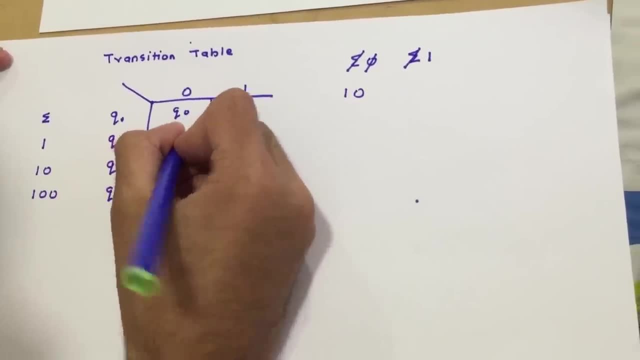 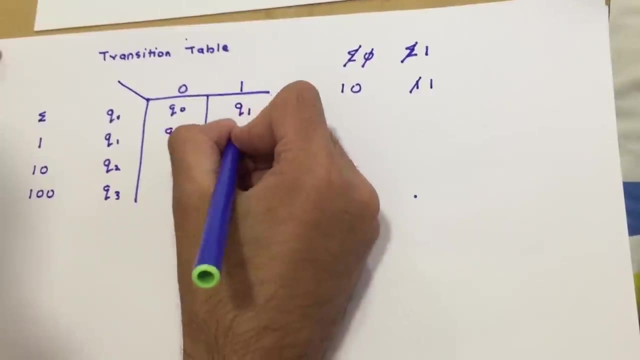 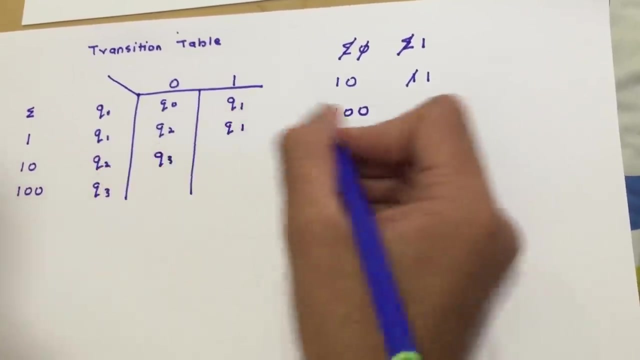 do I find 1 0 here? yes, so this will go to q 2: 1 1 1 1. there is no 1 1, so I'm going to cut this. 1. yes, q 1 1 0 0 is 1 0 0 present. yes, so it's going to go to q 3: 1 0 1 is 1 0 1 present, no. 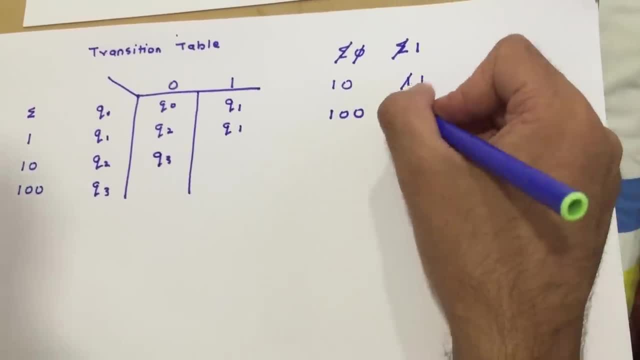 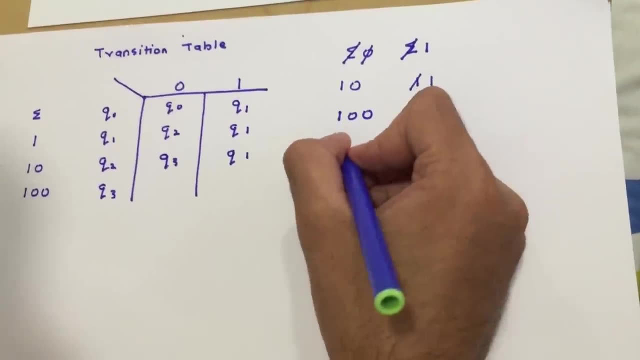 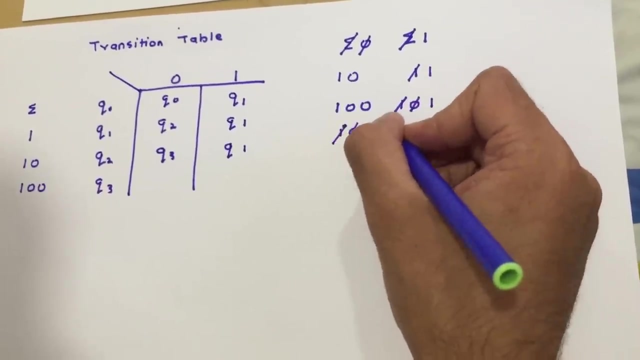 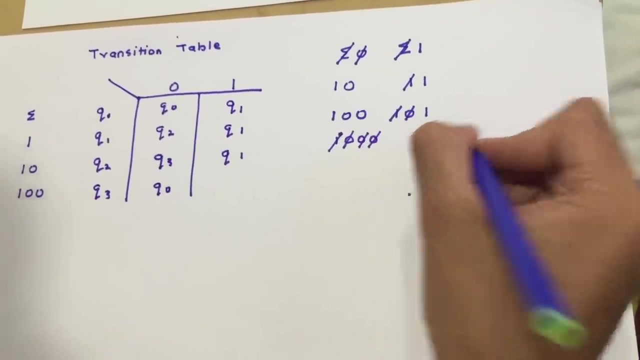 cut is 0, 1 present. no, cut is 1 present. yes, so it's going to go to q 1. similarly, 1 0 0, 0, not present. so I'm going to cut this. not present, not present, not present. so I'm going to send this to q 0 and 1 0 0, 1. 1 0, 0, 1 is not. 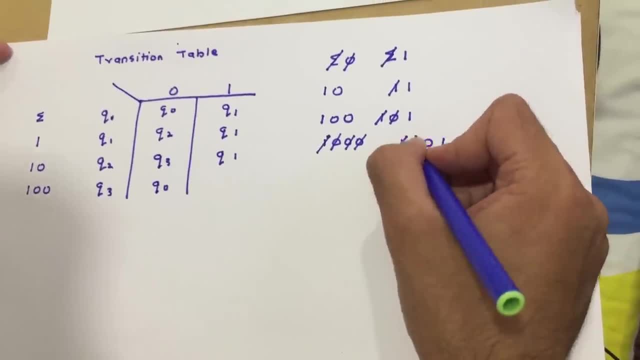 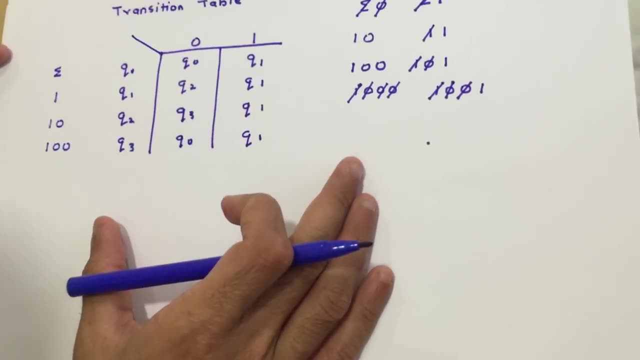 present. so I'm going to cut this: 0 0, 1 not present. not present, but one is present, so I'm going to send this to q 1 present. so I'm going to send this to q 1. so this is our transition table and looking. 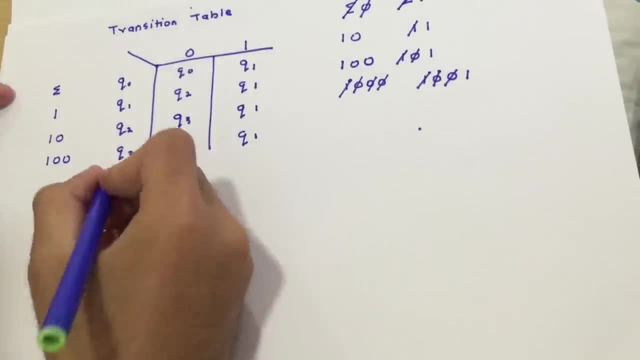 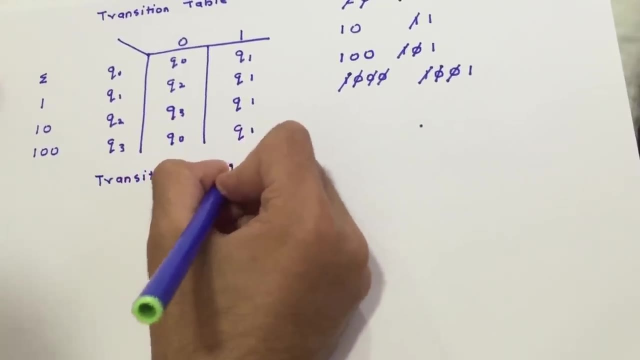 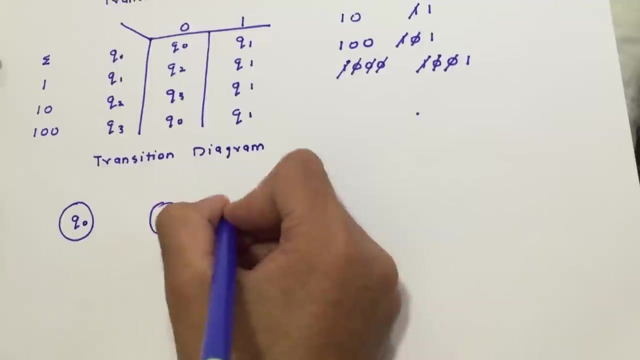 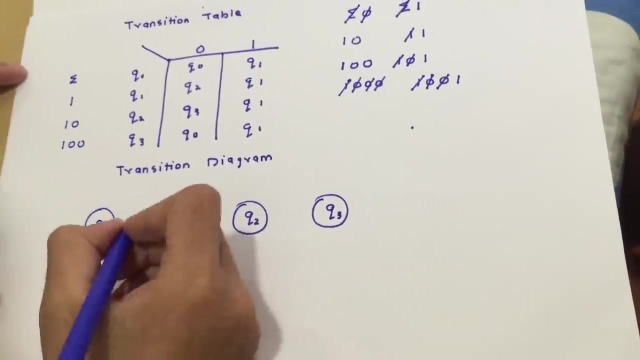 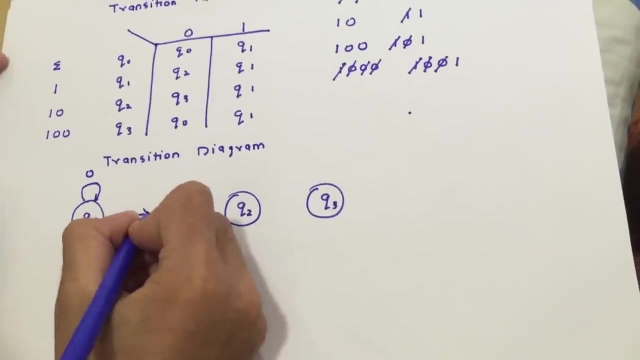 at the transition table. we are going to make a transition diagram, so I'm just going to make q 0, q 1, q 2 and q 3. so on 0, this goes, stays in the same state. on 1, it goes to q 1. similarly q 1. on 0 goes to: 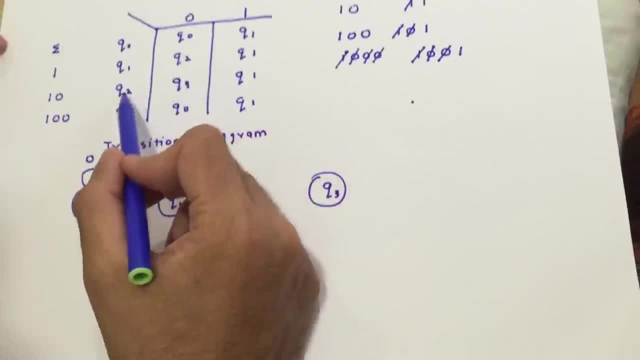 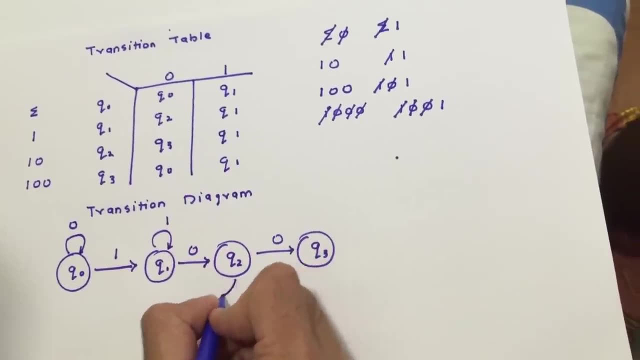 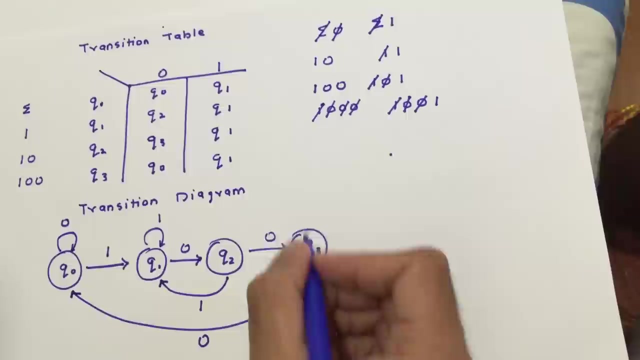 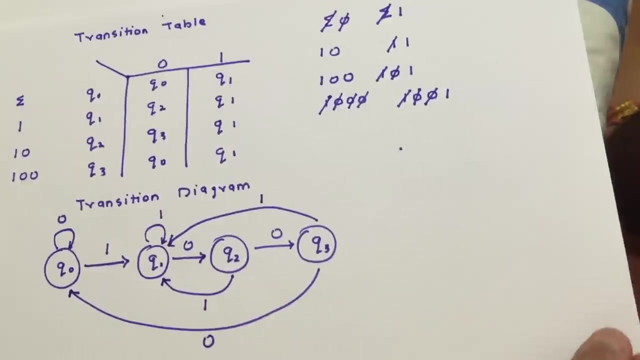 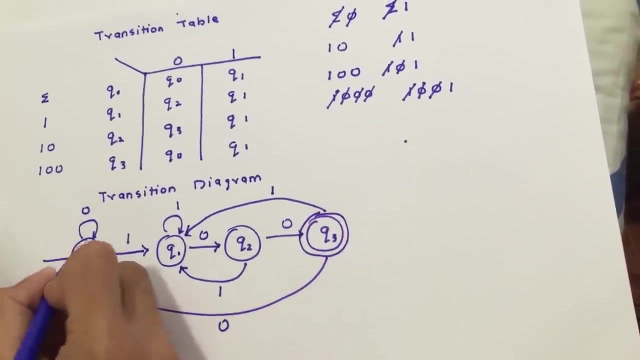 q 2. q 1 on 1 remains in q 1. q 2 on 0 goes to q 3. q 2 on 1 goes to q 1. q 3 on 0 goes to q 0. q 3 on 1 goes to q 1. q 3 on 1 goes to q 1. okay, so q 3 is our final state. this is our. 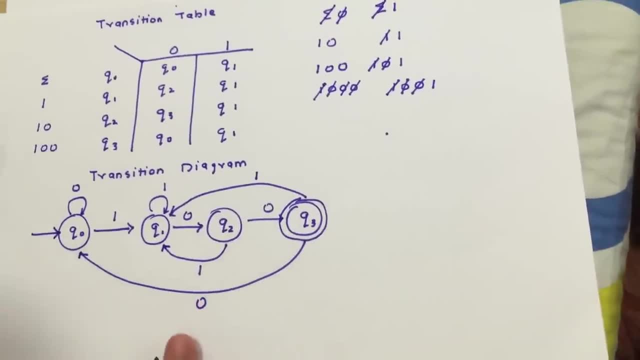 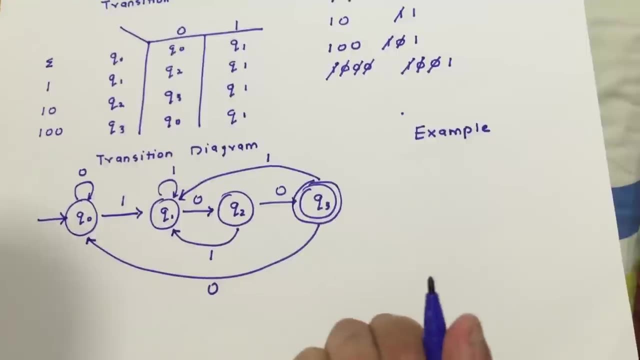 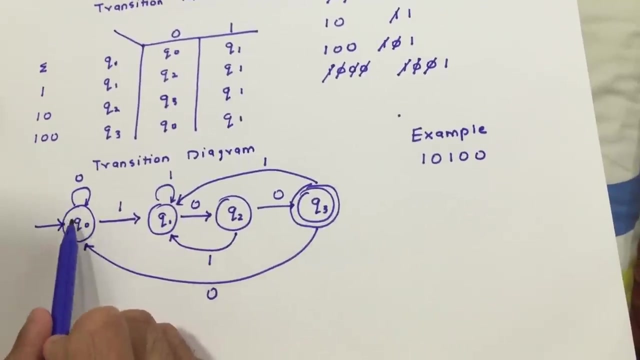 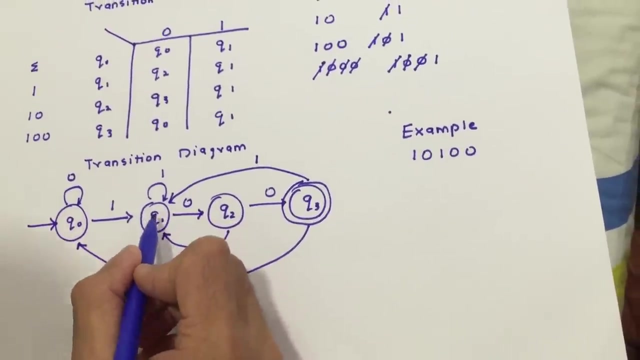 initial state. now how do we check if our diagram is right? so I'm going to take a small example and verify. so let us consider any string ending with 100, for example, one zero, one, zero, zero. So our initial state is q0. So first, when 1 comes, it will go to q1, then when a 0 comes, 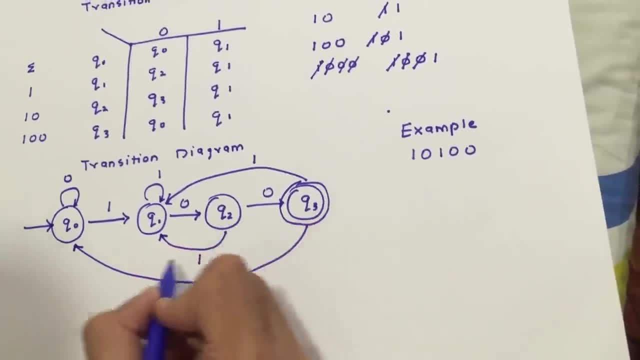 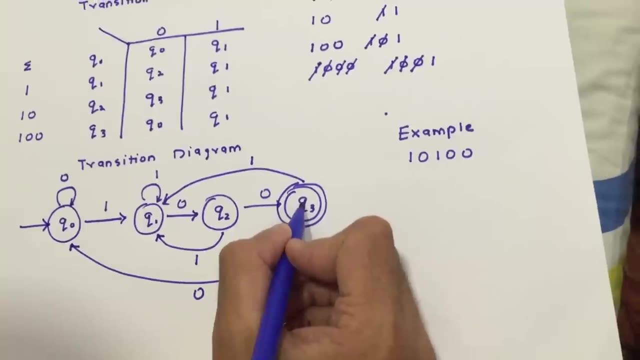 it will go to q2, then when a 1 comes, it will go to q1, then when a 0 comes, it will go to q2, and again, when a 0 comes, it will go to q3.. So our string is ended and since q3 is, 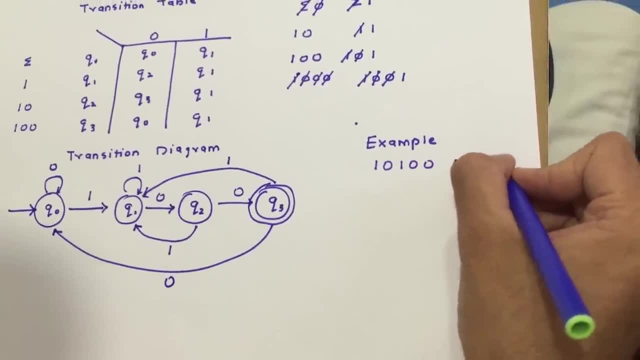 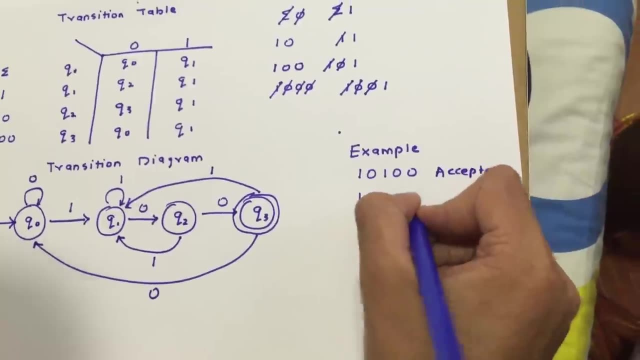 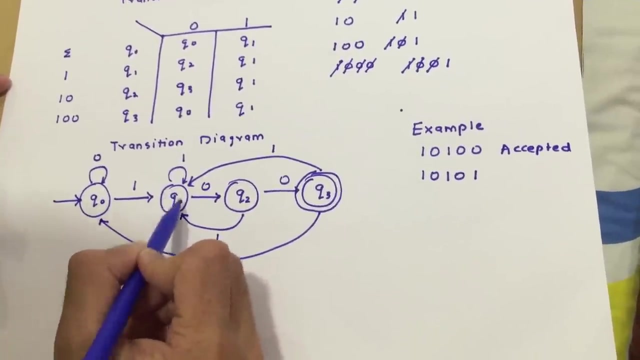 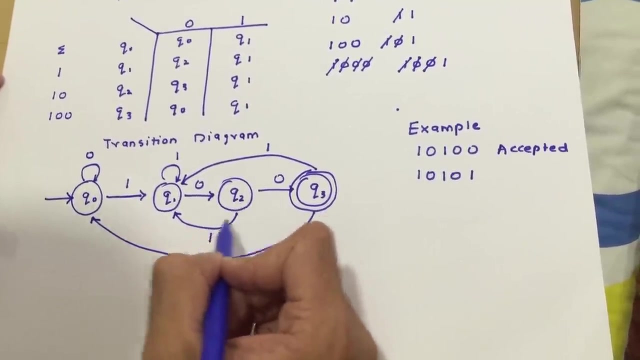 our final state, this will be accepted. Let us consider another string which does not end, for example 1 0, 1 0, 1.. So, similarly, initially we had the q0. So on 1 will go to q1, on 0 will go to q2, again, on 1 will go to q1, on 0 will go to q2, but on 1 will.